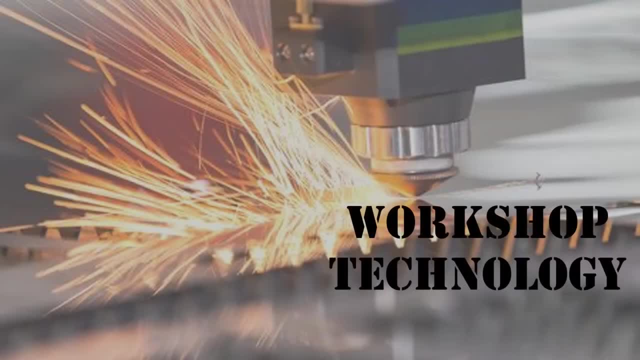 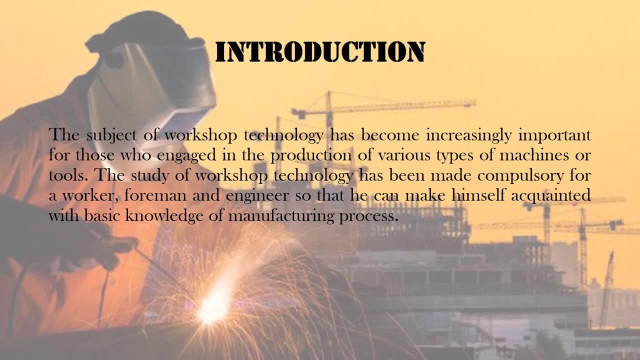 Hello friends, in this video we are going to learn some basics about the workshop technology. Let me give an introduction to the topic. The subject of workshop technology has become increasingly important for those who engaged in the production of various types of machines or tools. 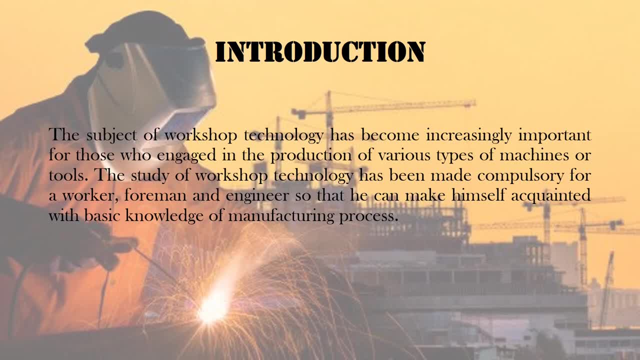 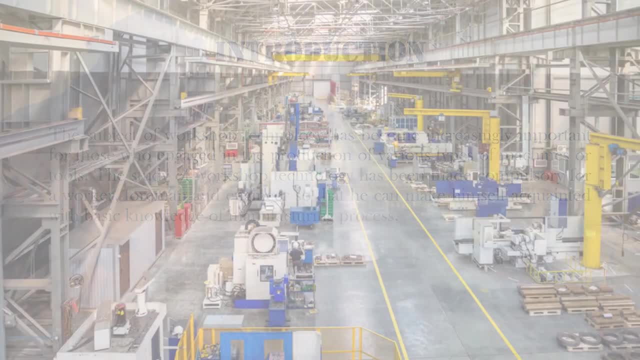 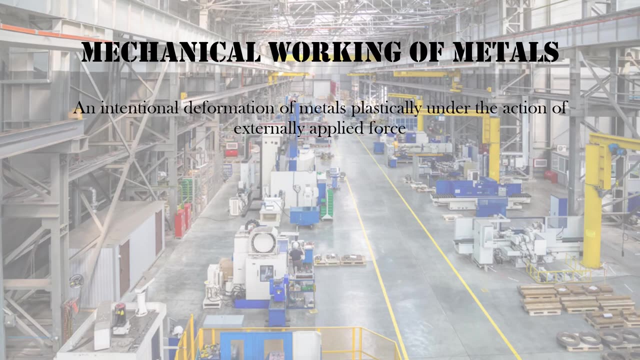 The study of workshop technology has been made compulsory for a worker, foreman and engineer so that he can make himself acquainted with basic knowledge of manufacturing process. Now, coming to the topic, mechanical working of metals. It can be defined as an intentional deformation of metals. 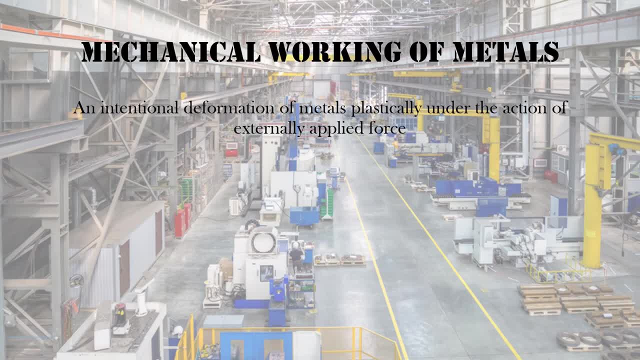 plastically under the action of an externally applied force. It can be classified into two. The first one is hot working, in which working temperature is greater than the recrystallization temperature of metals, And the second one, cold working, in which working temperature is less than the recrystallization temperature. 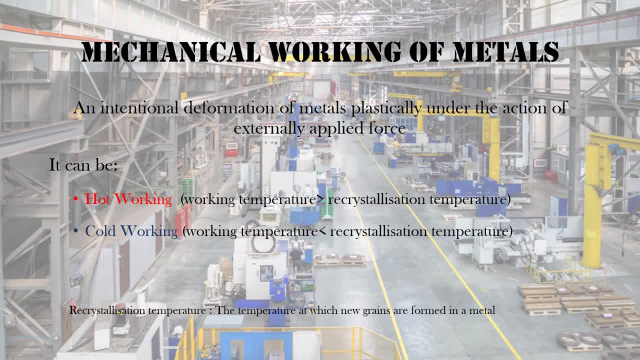 If you ask me what is recrystallization temperature, Then it is the temperature at which new grains are formed in a metal. Do you ever think why a metal is subjected to mechanical working? If so, the following are those purposes. 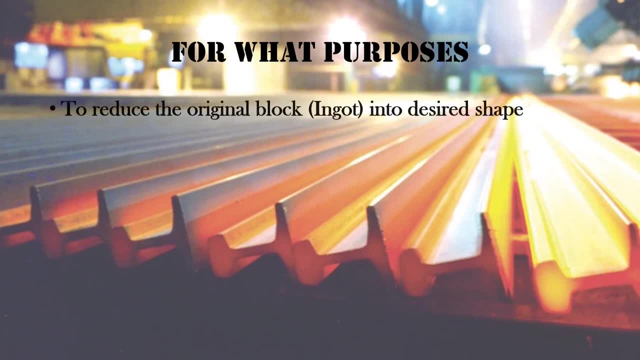 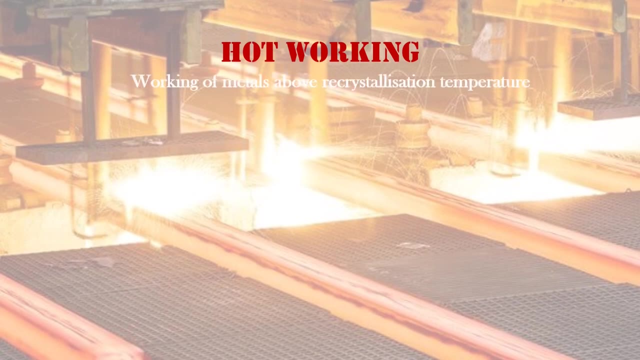 We use mechanical working to reduce the original block, technically called ingot, into desired shape, to refine the grain size and to control the direction of flow lines. Hot working Said before, it can be defined as working of metals above the recrystallization temperature. 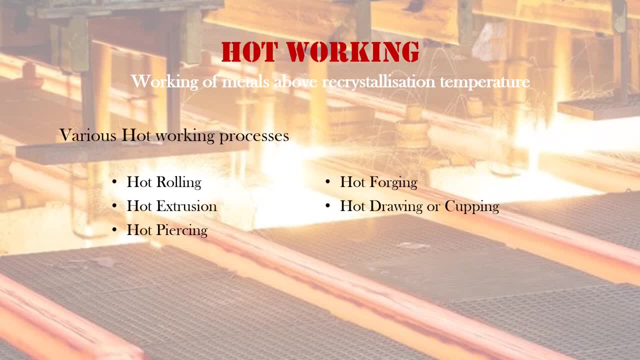 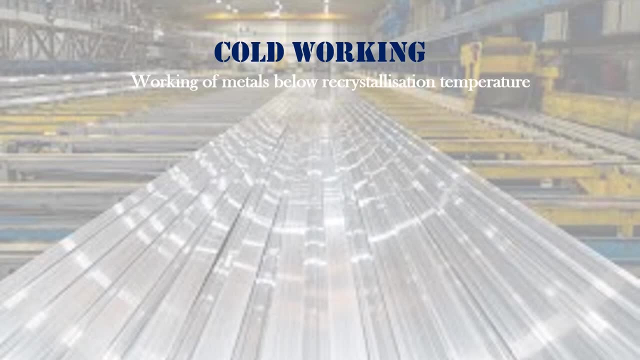 Hot rolling, hot forging, hot extrusion, hot drawing or cupping, hot piercing are various hot working processes. Cold working: It can be defined as working of metals below the recrystallization temperature. Cold rolling, cold forging, cold extrusion, cold drawing, cold spinning, cold bending, shot peening. 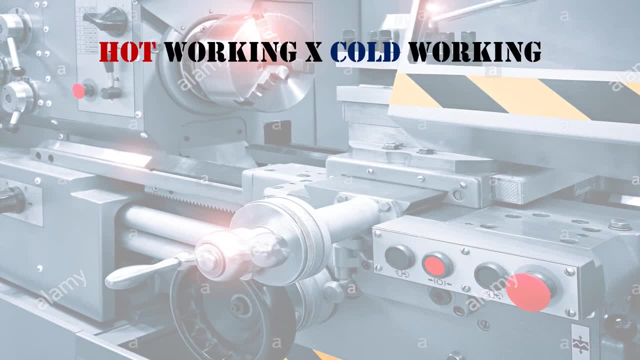 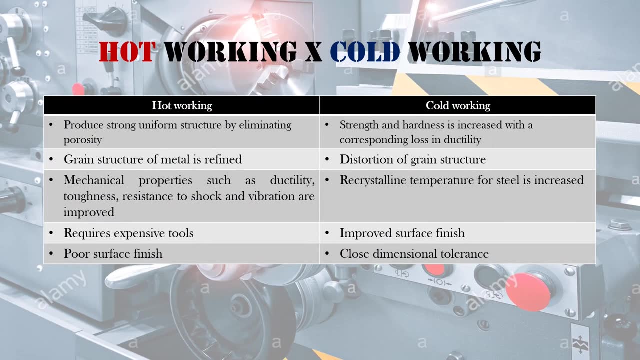 are various cold working processes. On comparing both, we can find that both of them have advantages and disadvantages. In the case of hot working, Mechanical properties such as ductility, toughness, resistance to shock and vibration are improved. Grain structure is refined. strong, uniform structures are produced.